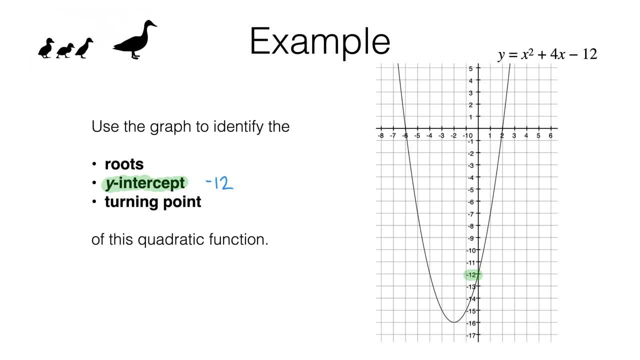 on one side is positive and the gradient on the other side is negative. and for this curve you can see that the turning point is right here. to the left of that turning point you can see we have a negative gradient. the curve is going down. and then to the right of that turning point. 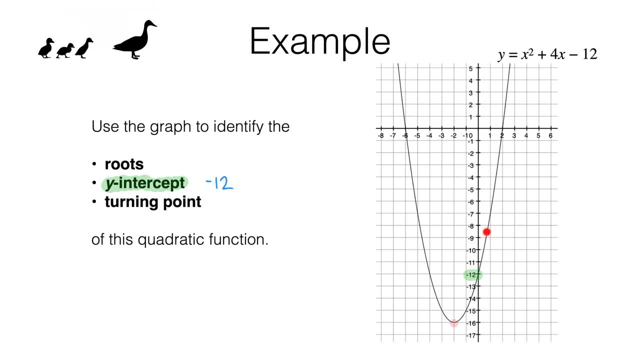 you can see we have a positive gradient. You can see the curve going up. Now for a turning point. what we're actually looking for is the coordinates of the point. So we have negative 2, negative 16 as our turning point. I'll just colour code this in red to match the diagram and we can now move. 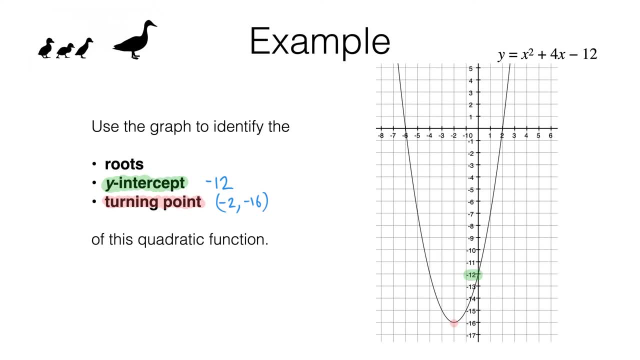 on to roots. Let's go back to our function. We have the function x squared plus 4x minus 12.. That is a quadratic function in x. The roots of that function are simply the values of x that make this equal 0.. What possible values of x do we need to substitute into here and here? 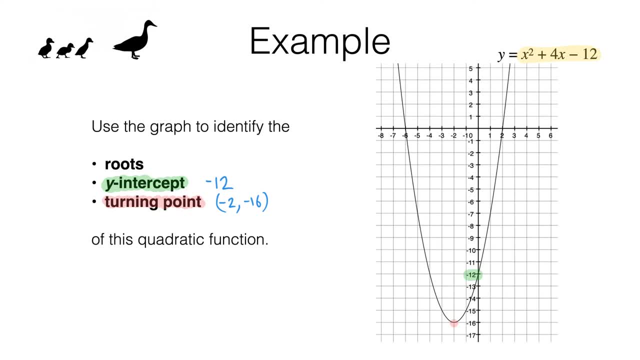 so that this gives us an output of 0?? Well, the answers are simply the x-intercepts of the curve. It's where the curve crosses the x-axis and you can see that happens at negative 6 and 2.. So our roots are simply negative 6 and 2.. 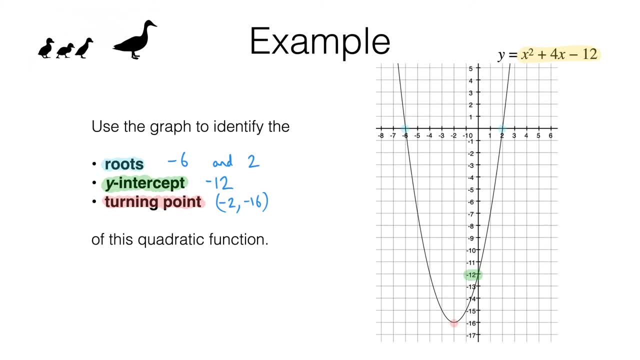 We can test this for ourselves. Let's take 2.. When x is 2,, if you substitute that into here, you'll see we get 2 squared, which is 4.. Then we need to add on 0.. 4 times 2, so that's 8, and then we need to subtract 12.. 4 plus 8 minus 12, that gives us 0.. 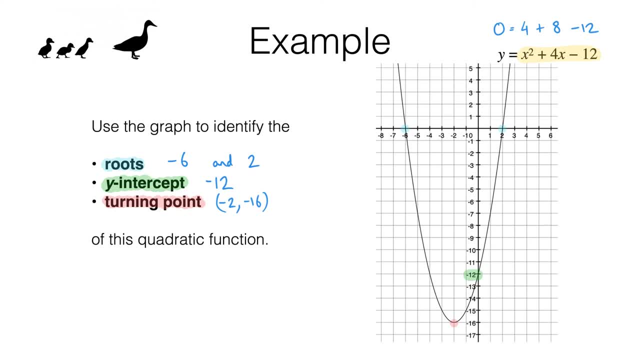 And that meets the definition of a root. Remember, when you substitute a root into a function, you get 0.. Also, notice how this fits in with what we understand about plotting graphs. Remember this is the graph of y equals x squared plus 4x minus 12.. 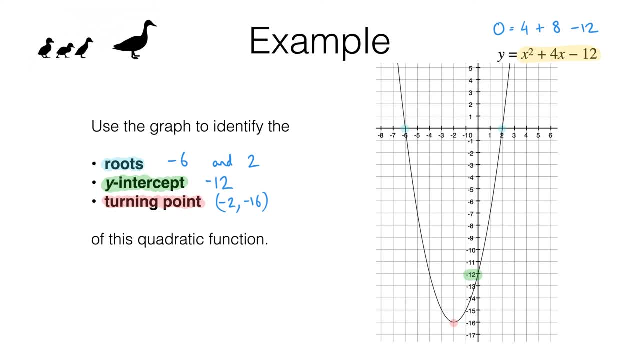 And when we do that we get 0. So we get 0.. When we substitute 2 into here, we get a y-value of 0. So that tells us that 2, 0 is a point on the curve When x is 2, y is 0..